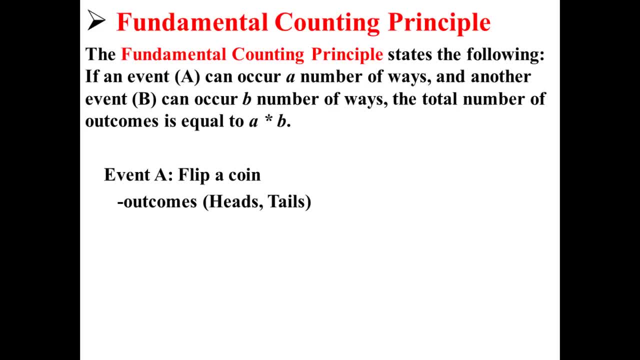 Here we have event A, which is flip a coin. When you flip a coin, there are two outcomes, heads and tails. Event B is we roll a die. When you roll a die, there are six potential outcomes: One, two, three, four, five and six. 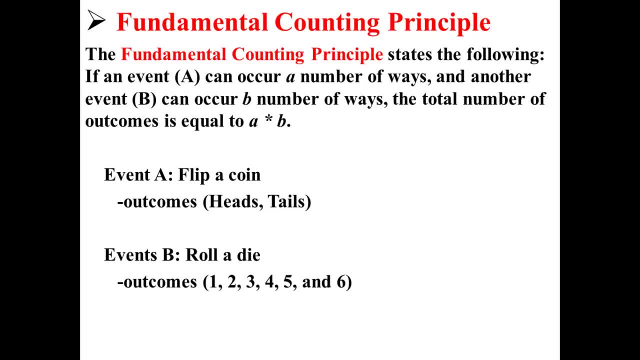 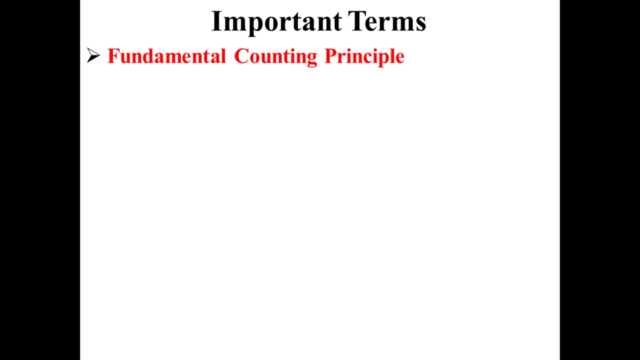 How many different ways can both of these events, event A and event B, occur when done together? Well, our number of possible outcomes is equal to A times B, which is two times six equals twelve. If we perform event A and then event B, there are twelve different numbers of possible outcomes. 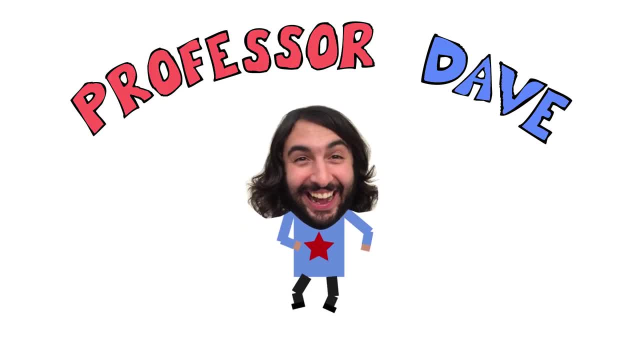 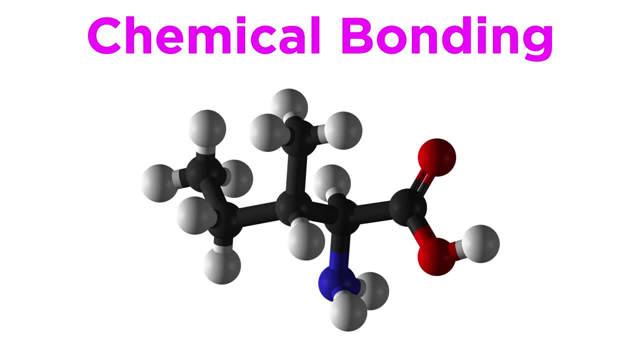 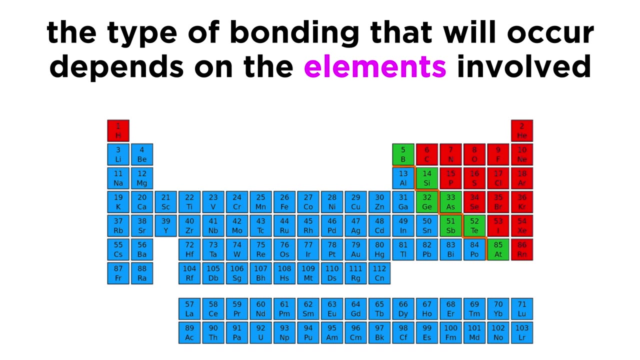 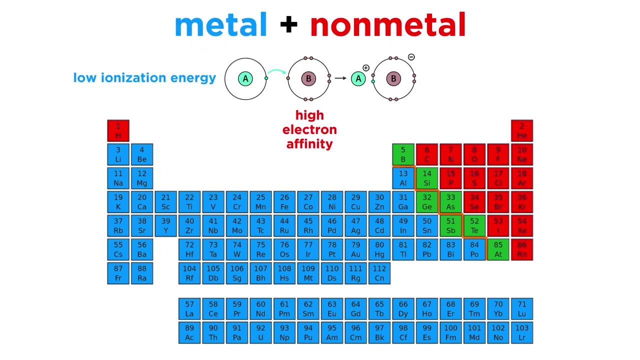 Throughout this general chemistry series, the phenomenon of chemical bonding has been a primary focus. We know that there are different types of chemical bonds, and the kind of bond that will form between atoms of two elements depends on the identity of those elements, If one element has a low ionization energy and the other has a high electron affinity. 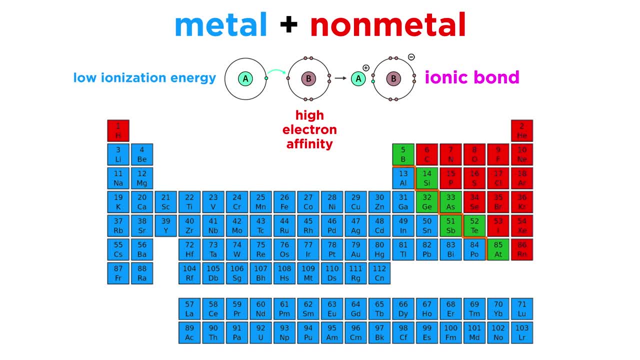 electron transfer will occur, resulting in ions which will then interact via ionic bonds. So, for this reason, a metal and a non-metal will tend to make ionic bonds due to their positions on the periodic table, By contrast, two non-metals being from this region in. 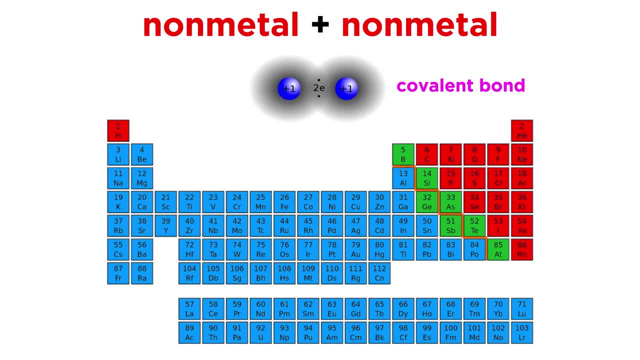 the upper right section of the table, will tend to share electrons to make covalent bonds. The same can be said for a metalloid and a non-metal. again, covalent bonding will be most likely. But what occurs between two metals? What kind?